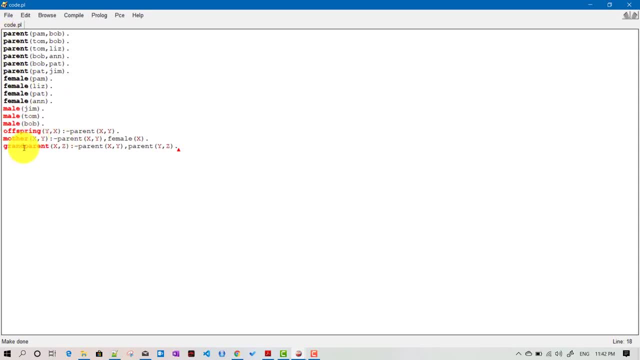 facts and a lot of rules over here, right, corresponding to offspring, mother, grandparent, those kind of stuff. Okay, Let us try to introduce a new concept. Okay, And let's see how we can define that rule in prologue. Okay, I just wanted to set up the ground for the 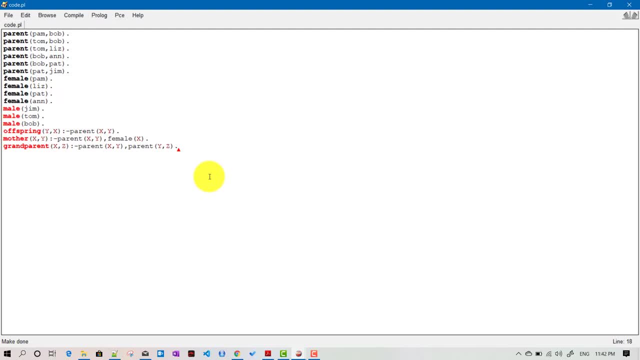 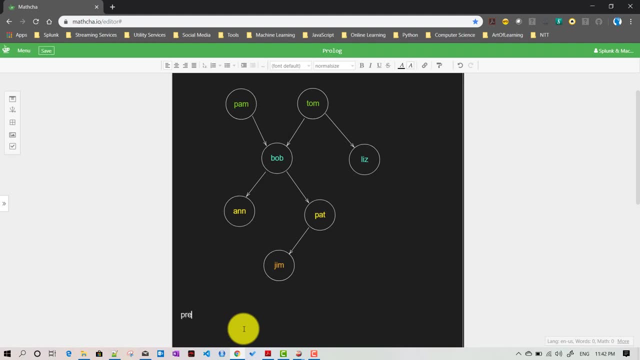 recursive definition of the rule. So for that, what we'll do is we will try to see a, we will try to create a new rule called predecessor Okay, predecessor, Okay. So now, if we think about this particular relation, so relation over here, okay, there are. there are two cases. 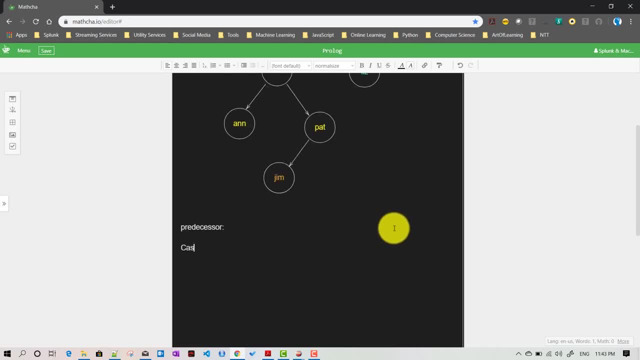 coming up in our mind: Case one, let's, let's write it about this, Case one and case two. Okay, Now, case one could be very simplistic case where a parent is all it's always a predecessor of this, of its child, right? That means, if I just talk about 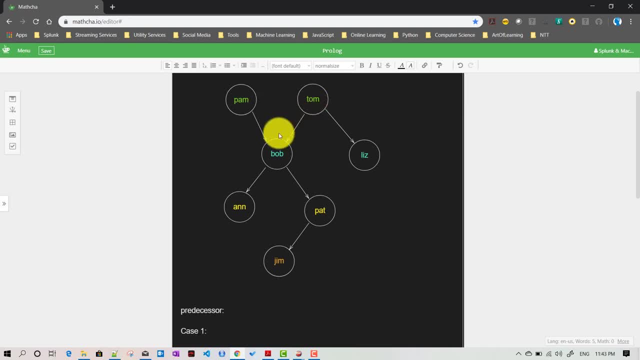 Tom and Bob over here. Tom not only the parent of Bob, it also the predecessor of Bob as well. right Now, let us, let us try to see this particular chain over here: Pam, Bob, Pat and Jim. Okay, Now, if you. 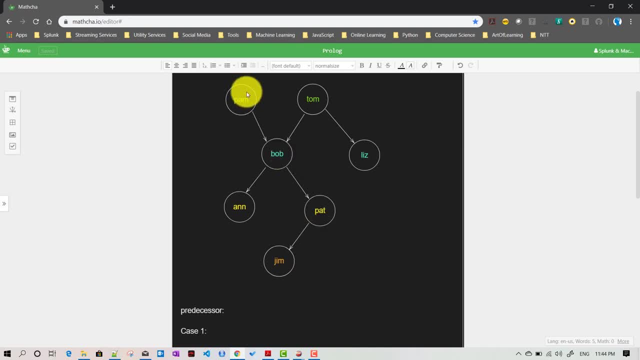 see it over here for Jim, Pat, Bob and Pam- all are predecessors, right? That means when I, when I talk about parents of parent, right, those are, those are predecessors as well. Okay, so case one, we are talking about case one, we're talking about a relationship, something like this: for all, for all x. 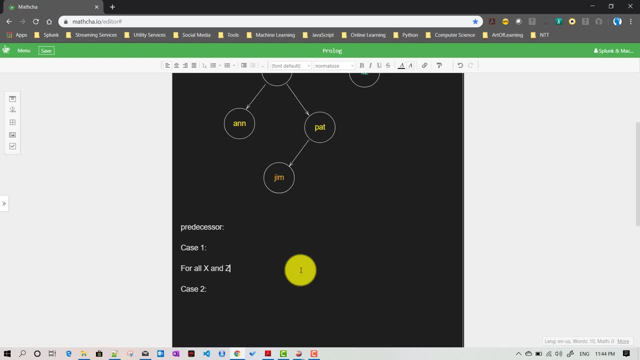 and z. Okay, So if x. so x is a predecessor, okay, of z. if x is parent of z, right x is parent of z. this is the simplistic case we are talking about Now. case two is, if I just write in in, in terms of mathematical logic: 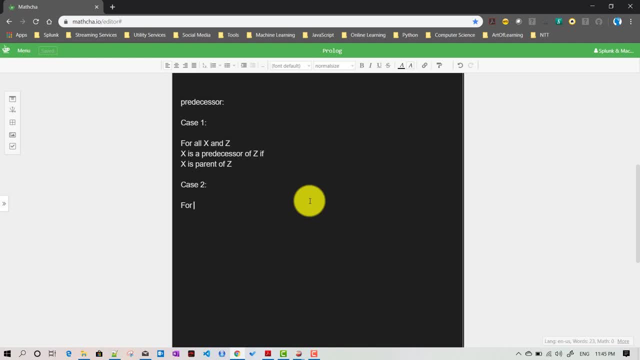 So for all x and z, similar way, okay, x and z, okay now x is predecessor of z. so if i just just copy this this line over here: okay, x is predecessor of z. if, if let's say, let's give it a name over here, okay, see, if x is parent of z, okay, x is parent of. 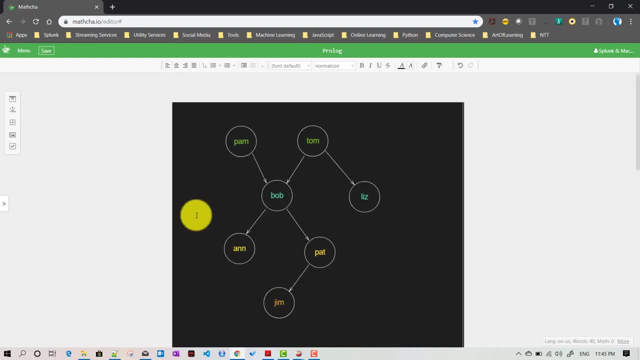 y, okay, that means there is a y if i, if i just go back to our diagram over here, we are talking about the predecessor of gym over here, right? so that means, or let's say we are asking this question: is pam is predecessor of gym, right? which is essentially true, right? 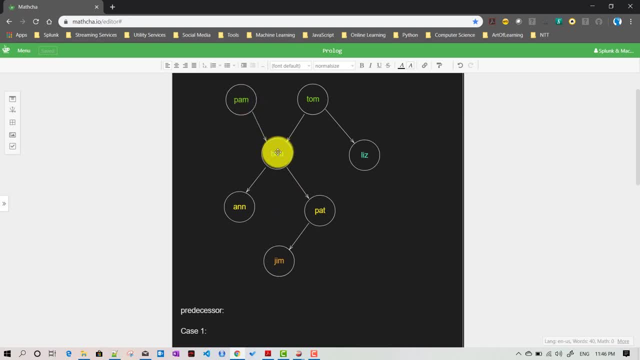 so that means we are basically talking about: there is a y okay where x is parent of y okay and y is predecessor of z here here, x is our pam and z is gym over here, right, that means we are finding a guy who, who is basically child of x over. 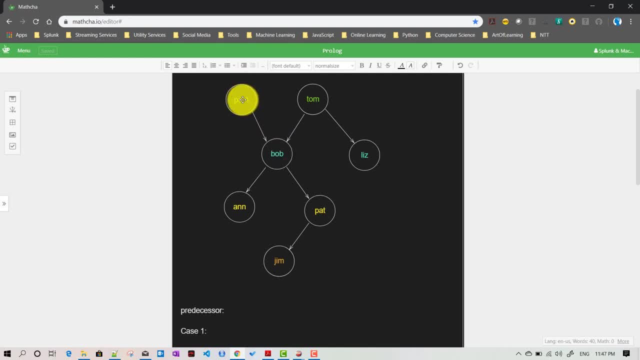 here. that means x is parent of that y over here, right, we are finding a third person over here who, where x is parent of that guy, okay, and y is the predecessor of gym over here, right, because between bob and jim there is another guy called pat over here, right? 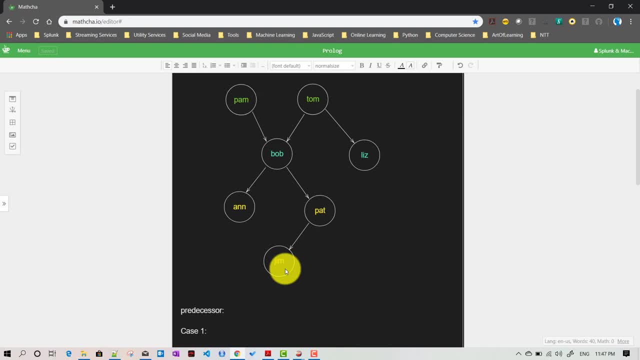 if you see it this this way of defining something, right? so let us first write it down over here. okay, so x is parent of y. that means we are finding a guy where x is parent of y and and y is predecessor of z over here, right? so this is. this is important. now, if you see it over, 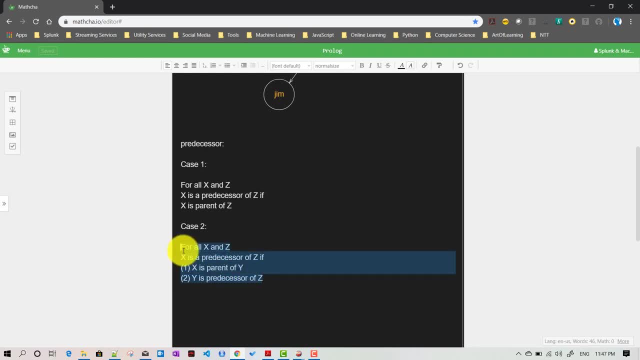 here in the in the second way of defining the predecessor relationship right. the second case: we are basically talking about the predecessor keyword itself, when, when we are defining the rule right, when they define the rule body over there, right, so so let us, let us write it down, this, this two rules, in prolog terms. okay, so we will go to our. 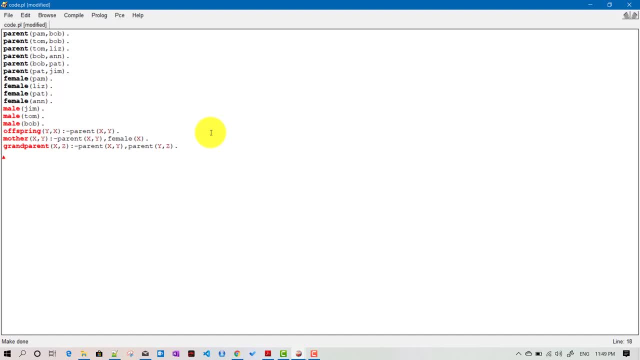 our same code base over there. okay, so we will write a rule called predecessor- okay, predecessor of x and z. okay, now here we will introduce another, another concept. let me write, let me write it down, these two rules first. okay, so this is how we are defining a rule: right, colon, then dash. 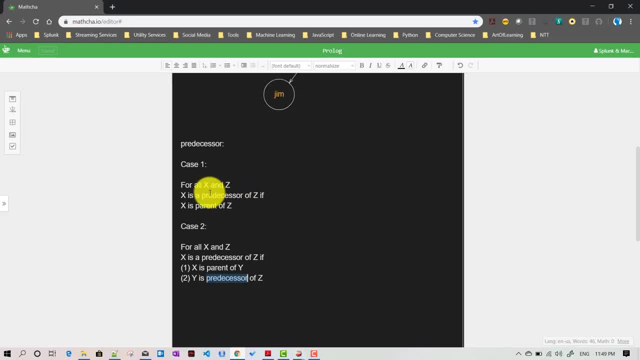 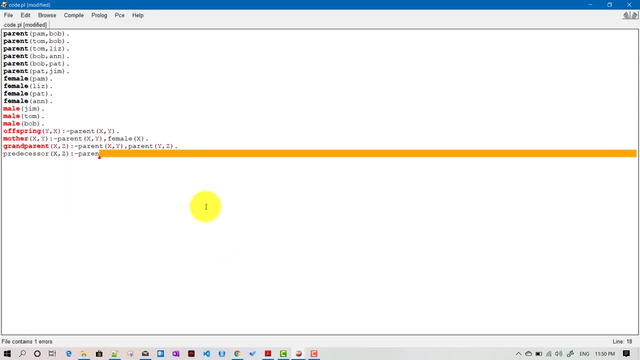 the dot, dot x in to the root of z over here. right now, what is? according to our first case, x has to be the parent of z, right? this is this is the first case. that means we are basically in the body of the rule. okay, parent of x, comma z over here. so this is the. this is the first case we are talking. 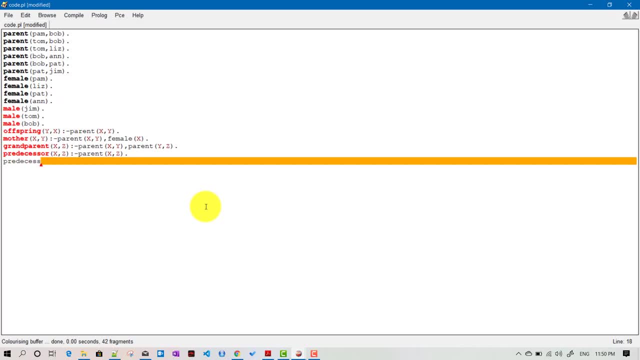 about right now, according to the second case. let us write it down now, if you see it, over here i am writing the rule name: same x, comma z here. okay, so colon dash. okay. now, if you see it, i am giving the same name because the relationship is same over here and this is this way of defining a relationship, where 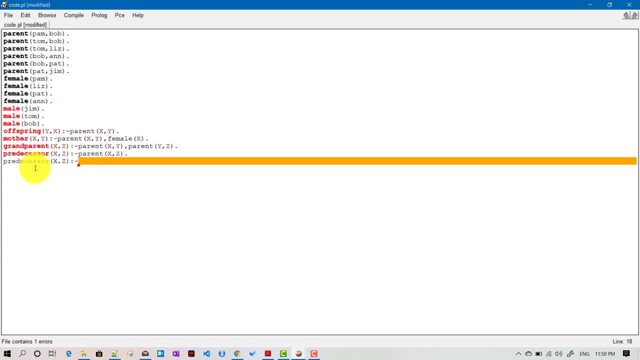 you have more than one clauses for a particular relation, called procedure as well. okay, but this is a some some terms we call it, but essentially we are defining more than one clauses for a particular relations over here. till now, whatever we have defined we, we have only single clause. 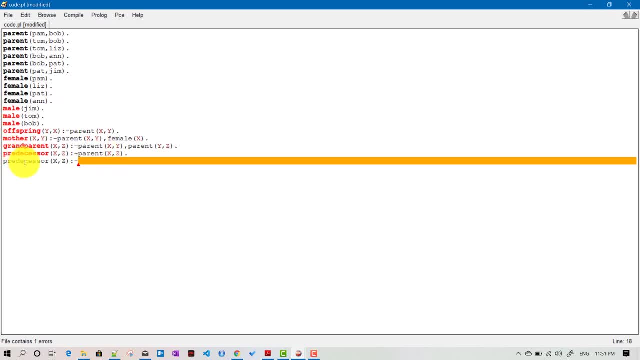 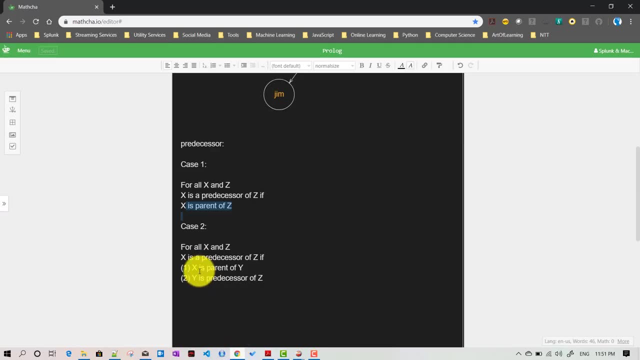 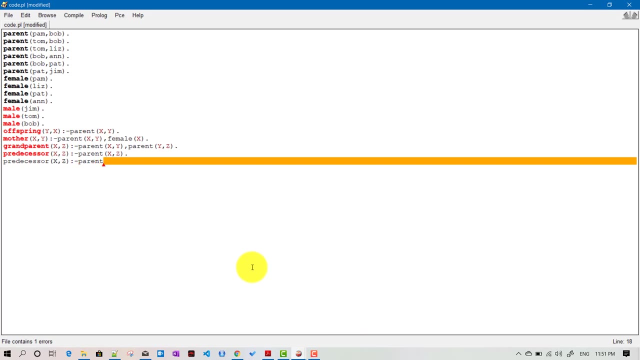 for a particular relationship. right now here we are defining more than one clauses over here. okay, so according to our second case, x will be the parent of y, right? so that means, if i just write it down over here: parent, so there is a y which is child of x, right, if i just talk about this particular relationship? 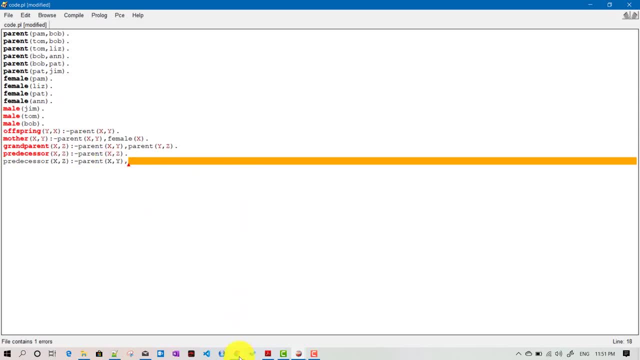 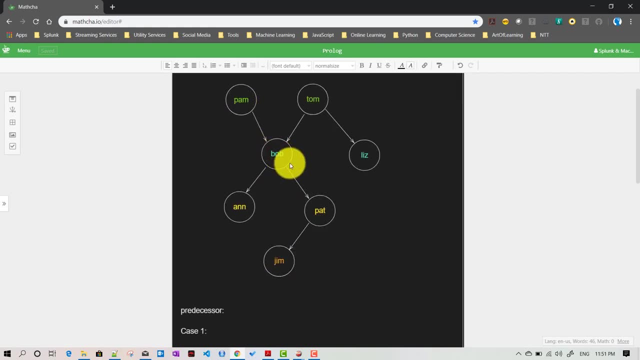 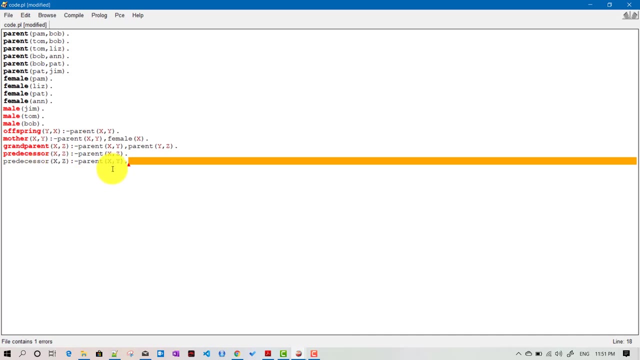 okay. and also y is the predecessor of z, right. so if our case z is zim and y is bob, right, that means y is also a predecessor of g, z over here. so let us copy this one or let's say: pretty predecessor, okay, so y is also predecessor of z over here. we will see, like, why this particular rule works. 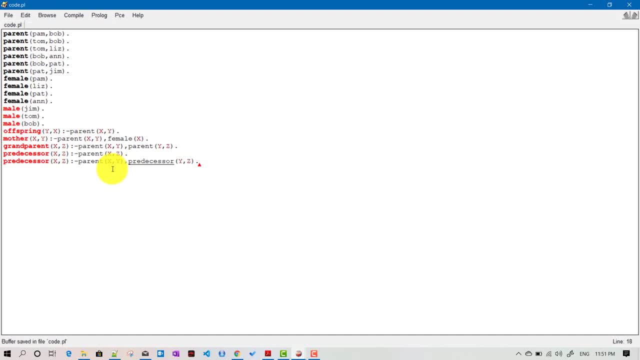 okay, we'll see that one. but but if you think about it like recursive way of writing a program is a very fundamental nature of computer programming, right? so that is what we are doing, it over here in the prologue, right? that means we are defining a rule. 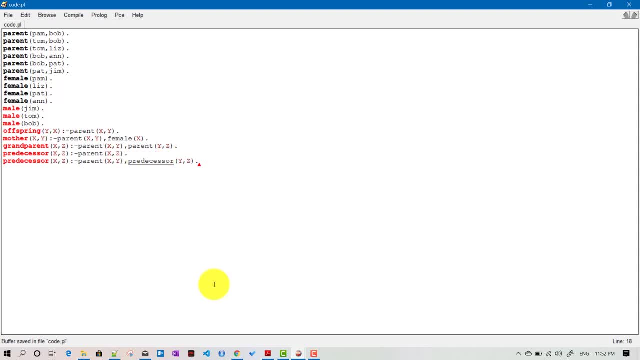 basically in terms of itself. over here, if you see it over here and and if you see it over here in the in the swi prologue, it is basically underlining this, this particular relationship name over here, right the predecessor, to show like it is, it is defining, defined in terms of itself, only that's the. it is showing. 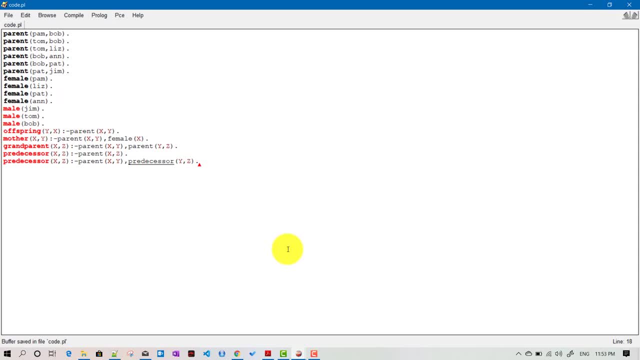 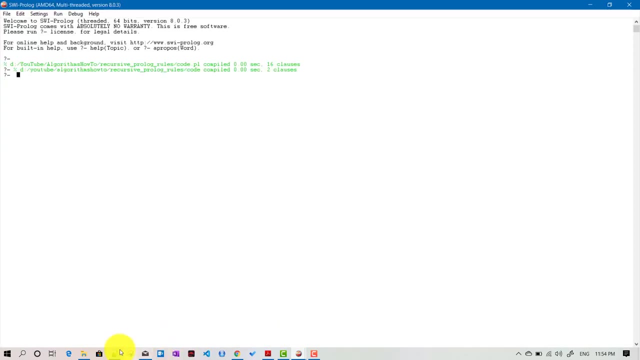 the recursion. basically, now let us first see whether whether this particular things works or not. then we will see why it is working. okay, so we will compile first. now we will go to swi prologue. now let us, let us, let us check it out in a check it out whether a simplistic case works or not. okay, 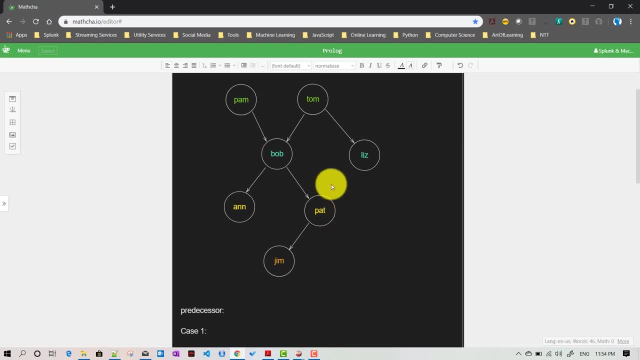 so we will. we will say like tom and pat. let's say okay, tom, or and also we can, we can do anything is fine. okay, so we are asking a question to prologue: whether tom is predecessor of pat or not. okay, it's very simplistic question, right? so let us try to. 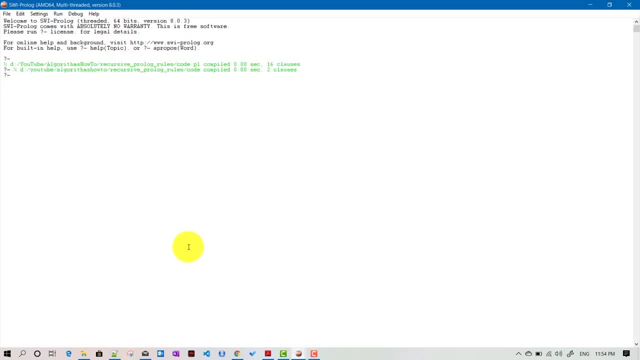 let us see what prologue is saying: okay, so we will call, we will give a goal, call something like this: pre this sir, okay, we will. the first argument is tom and the second argument is, let's say, pat. okay, so, let me, let me try to see tom and pat. yeah, so if i just call this one, 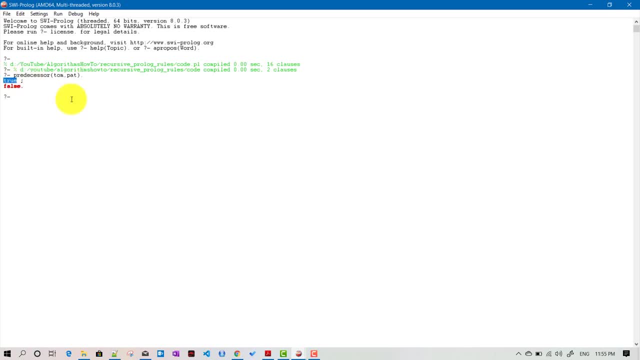 let me just call this one. so if i just call this one, okay, if you see, prologue is saying true over here, so that means our, our rule, our rule has been working over here. now let us see why it is working okay. so basically, we asked this question, right. 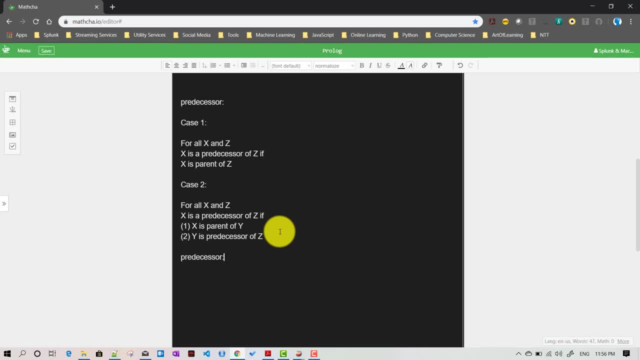 with this particular goal over here, right so, predecessor, tom comma, pat, right so we are basically talking about this, this particular chain over here, right so now. so we, we asked this particular question now, if you see, we, for predecessor, we have defined, we have defined two rules over here, right one is the predecessor. 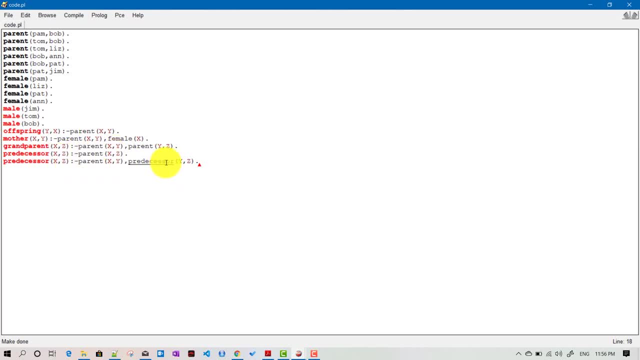 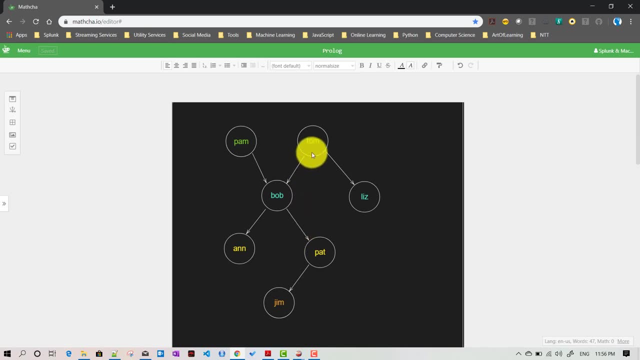 which is the direct parent and the predecessor in terms of itself, right now, when i talk about tom and pat. okay, now prologue will try to find something like this one: now tom is parent of bob, right. so now, if i just, if i just write it down over here: 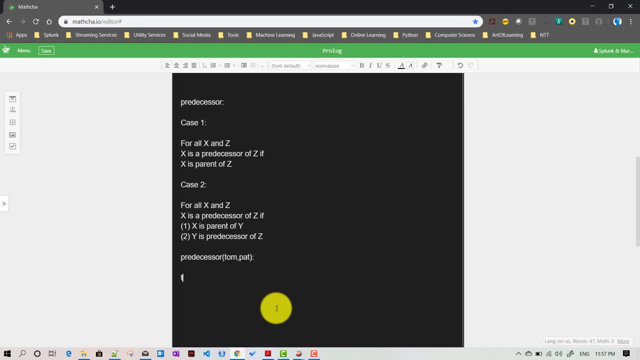 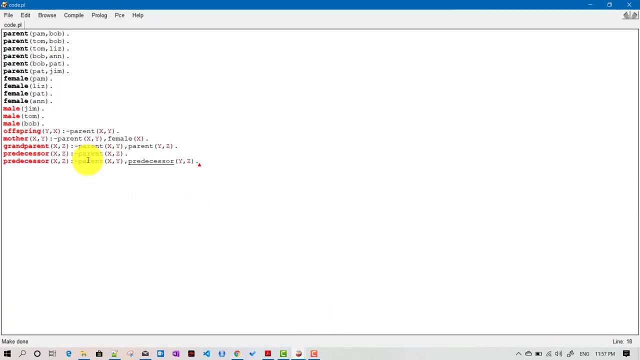 according to the case number one, to, if i just say, parent of tom, comma bob, okay, because there is a y involved over here. okay, so now this is, this is a fact. right, because tom tom is parent of bob. parent of bob, now this is also defined over here. right, because if i, if i just, if i just see, like 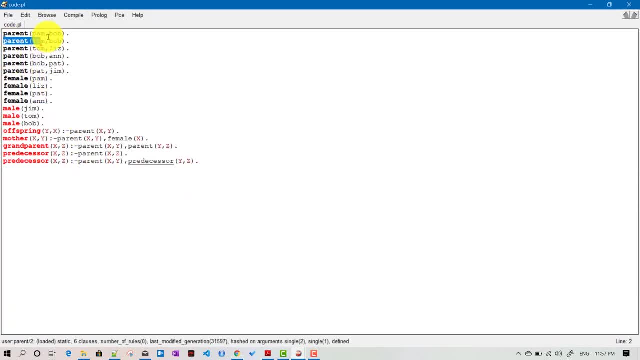 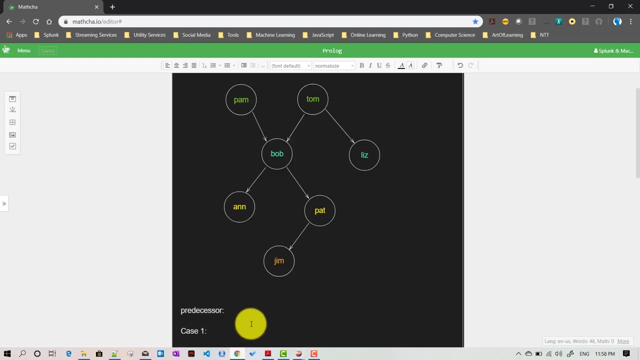 this, this particular rule, because when prologue is answering the question, right it is. it is basically consulting with all these facts and rule over here, right so tom is parent of bob. this is a fact over here which we have defined over here, right? so this is always true, right? so this is. 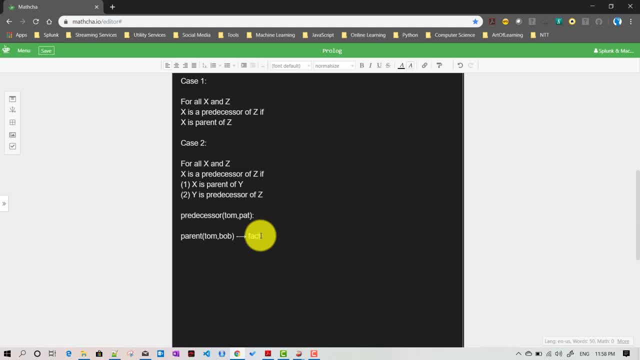 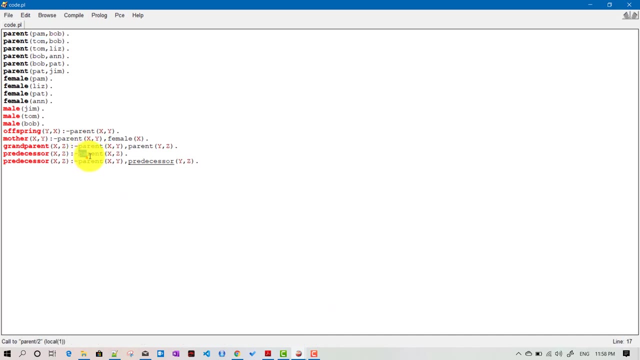 a fact. that means always true over here, right. so now, if this particular relationship is true, that means, according to the rule number one, if i just go back over over here again, so we, we, we already saw tom is parent of bob. over here, that means tom is predecessor of bob. that 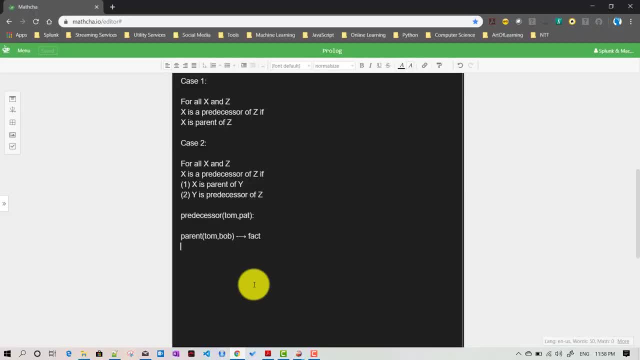 is also true. right, so we can. we can write something like this: so this does. this means predecessor. okay, tom is also predecessor of bob, correct? because of this fact, because this is fact and this is the body of this predecessor rule according to the first rule, right, so that means this is also true over here. right, so this is also true. 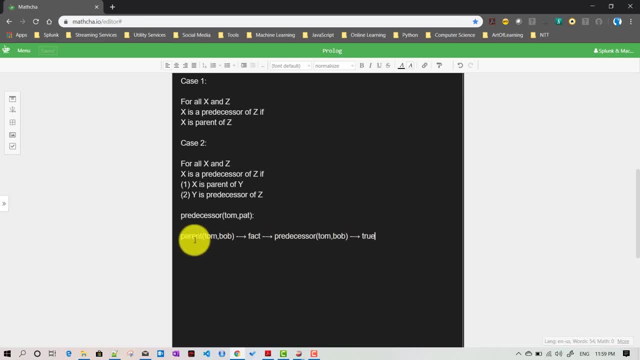 okay, so we, we established that parent of tom and bob means predecessor of tom and bob over here. now, let us, let us try to see according to the rule number two over here. okay, so if i, if i just go back over here again, according to the rule number one, so x is tom and z is pat over. 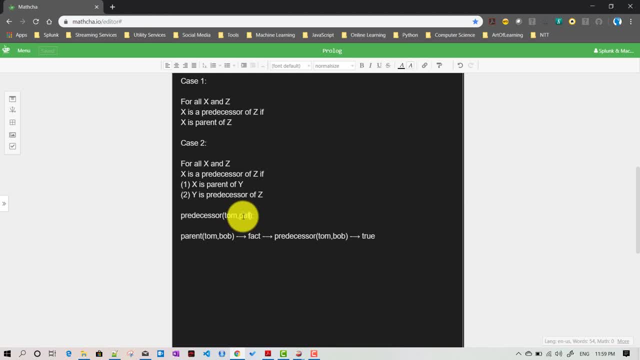 here, right? so as, as we already already seen it over here, we are passing, we are. basically, our main goal was to find it out whether tom is predecessor of pat or not, right? so in between we introduced bob over here, just to establish the fact that if tom is parent of bob, that means 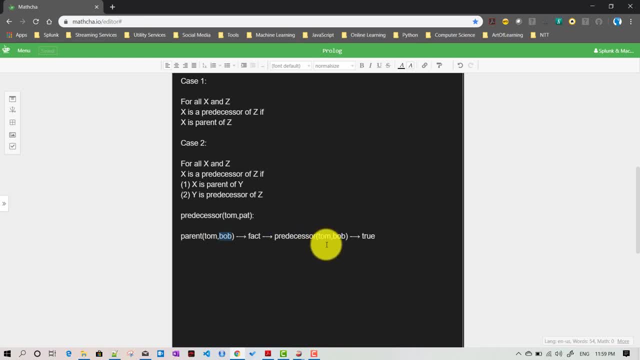 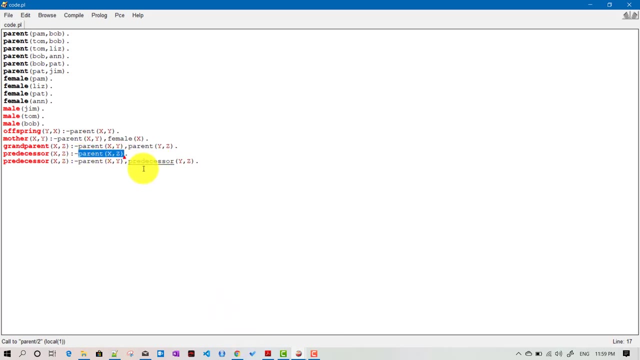 this predecessor, tom, is predecessor of bob as well. that is also true right now. if i, if i just write this particular rule, this particular rule according to the second definition, we have it right, the second line, we have it. so that means parent of x and y and y. here we introduce bob. because of that same reason, bob is our y over here, right? so if i just 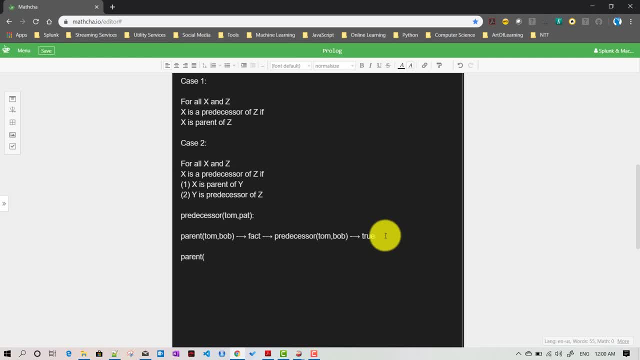 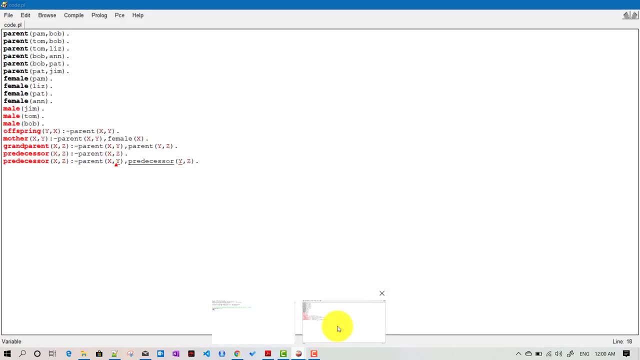 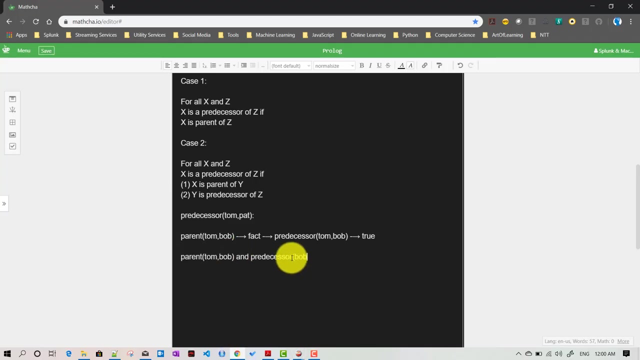 write something like parent: okay, tom, comma, bob. tom is our x, bob is our y over here, right. and predecessor: okay, now, predecessor, in the predecessor portion, what what we are sending? we are sending y and z, right? so our y is bob over here, correct, and our z is pat over here. 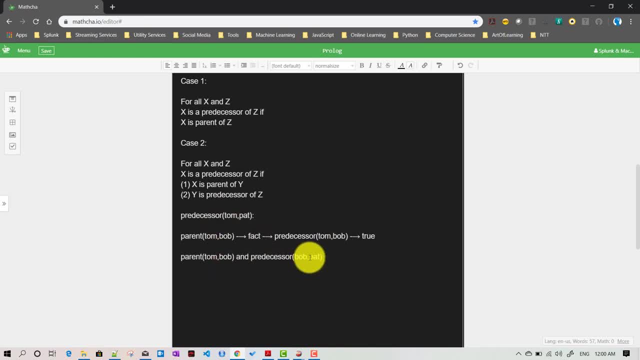 so now the rule is becoming something like this: now, right now, we already established: this guy is true over here, right now. let's, let's try to see whether this guy is true or not. if that is true, then we can directly say: tom is definitely a predecessor of pat. right now.